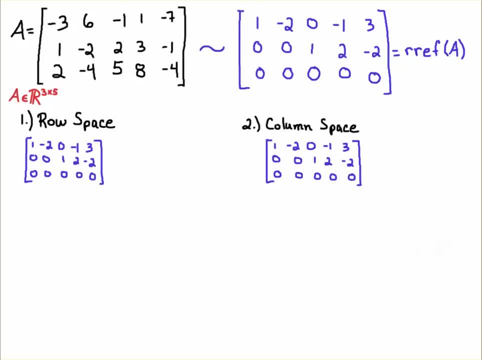 And then, once you have the RREF, it's actually just rather simple to identify what the row, what the row space and column space of the matrix is. For the row space, you identify the non-zero rows. For the column space, you identify the pivot columns. 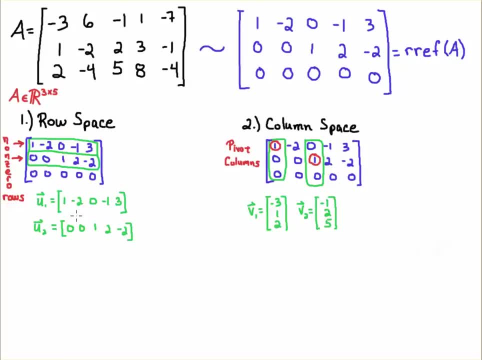 The non-zero rows for the row space will provide you the bases for the row space. So this top row here, this will be our bases, and this second row here, this will be another basis element and that'll be the basis for the row space. 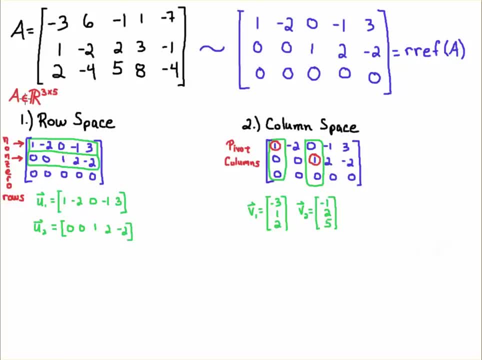 Notice that the matrix A is a three by five matrix with real entries. so we denote that by saying: A is an element of the vector space of matrices three by five matrices with real entries. so that's how we denote it: R- three by five. 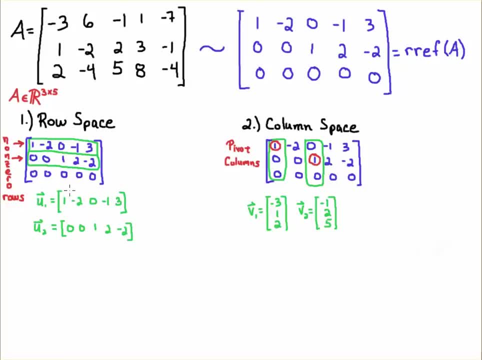 And it's a five-dimensional vector for the row space, each of the basis elements here. Now, because of the row operations, we can't relate without more information. we can't relate the row space necessarily directly back to the matrix A. However, with the column space we can, because 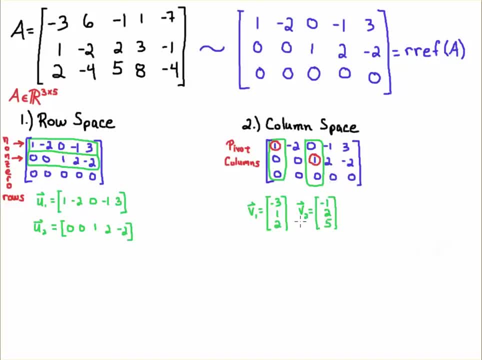 we typically don't swap columns. we may swap rows and such. so with the row space you just get down to the RREF and then you just look for the non-zero rows and you just pick those out and you're done for the column space. you look at the relationship here you have. 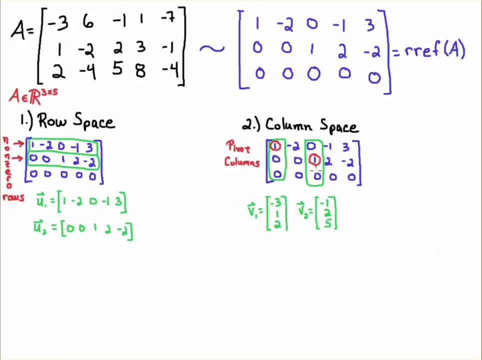 the first column and the third column of the RRF are your pivot columns. so you go back to your original matrix and you say the first column minus 3, 1, 2 and the third column minus 1, 2, 5 will be the basis vectors for your column space. so 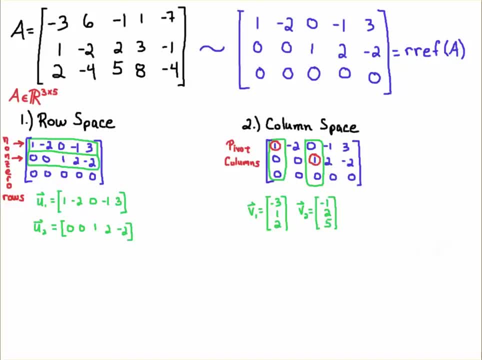 here you do relate back to the original matrix. so u1, u2 form a basis for the row space here and notice that they are five dimensional vectors. so there are. so the row space is a subspace of r5. if we call the RRF of a, if we call that matrix, if 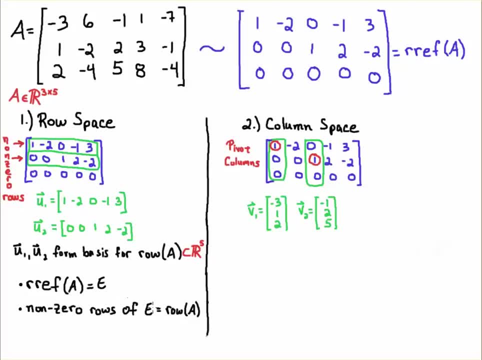 we call this matrix here e. then the non-zero rows of e give you the row space of a, which is denoted typically row of a. so let me summarize now the same thing for the column space. in the column space we have three-dimensional vectors. right, because this is a three rows to the matrix. so this column has three entries. 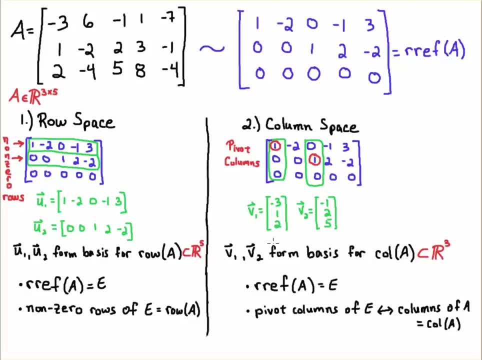 in it. so v1 and v2 form a basis for the column space of a, which is a subset of the vector space r3. and if we call the RRF of a, the matrix e, so we call this matrix e, then the pivot columns of e, they correspond to the columns of a. that 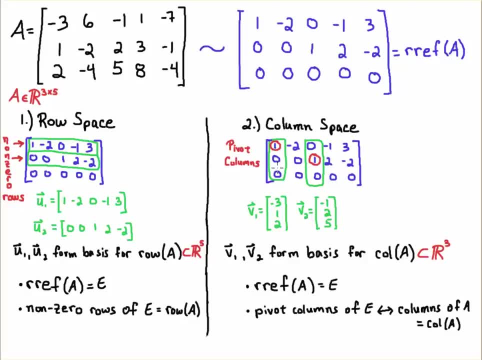 we call the columns of e column space of a. so you look. so for the row space, you just pick off the non-zero rows of e, which is your RRF of a. for the column space, you look at the correspondence between your pivot columns, so in this case column one and. 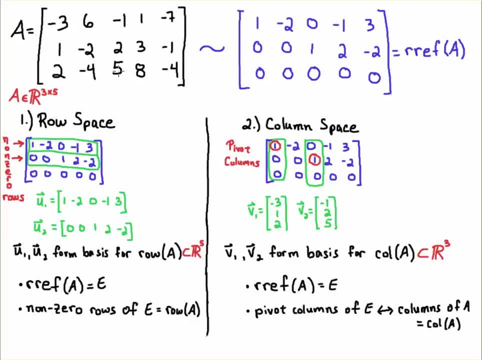 column three. you go back to the original matrix a. you pick off column 1 and column 3 and those vectors, column 1 and column 3, from the matrix a form your basis for the column space of a. so you pull off that invocative matrix and the column size becomes only 1 here. yes, and this where i've given rauszoh a. EF and a positive Evolut somehow, or. and that means the matrix a also has an equivalent column space B. The matrix has two spacers of bs for the column space o, 3 are between them: andhm, column Juan and calm three, Fabif 없 an Amith. the matrix a form your basis for the column space of a common 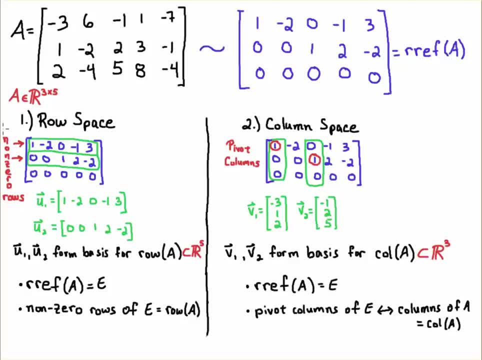 andhm of a usually denoted cow of a. now notice: in both cases, the number of basis vectors give you the row rank of a and the number of basis vectors give you the column rank of a, and in both cases the row rank of a is two and the column rank of a is two. 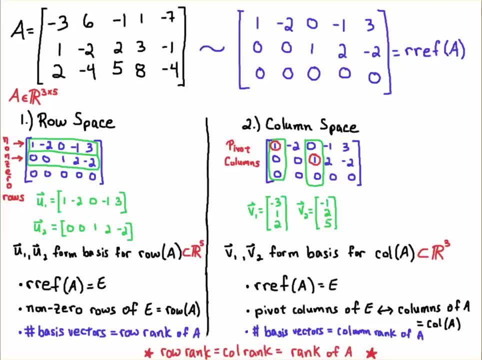 so there is a theorem. i'm not going to prove it now, but there is a theorem. you can look it up in your linear algebra text and it would notify you that the row rank is equal to the column rank and we call that the rank of a. 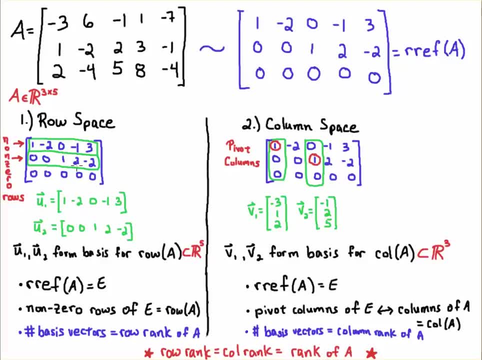 and so here's how you determine the row space and the column space of a matrix, and then, if you wanted to know what the rank of the matrix was, or the row rank or column rank of the matrix, in both cases doesn't matter- and also keep in mind the subtlety that the row space is a subspace of.